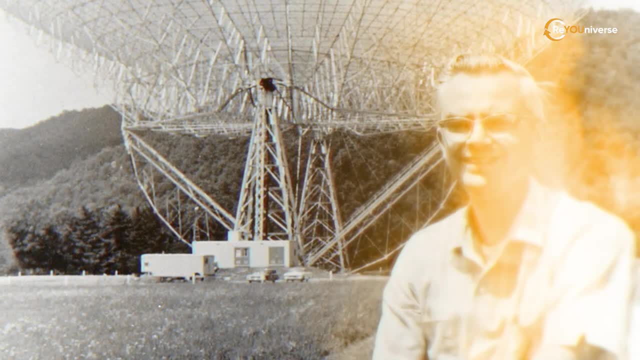 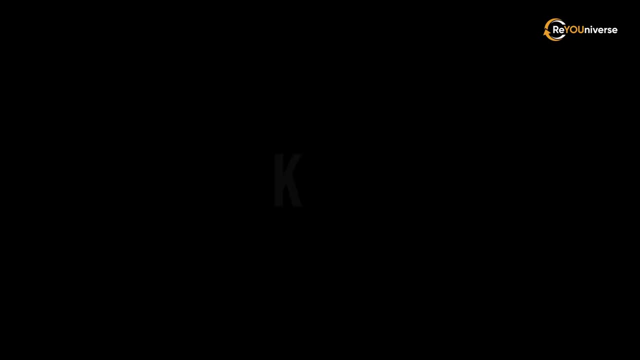 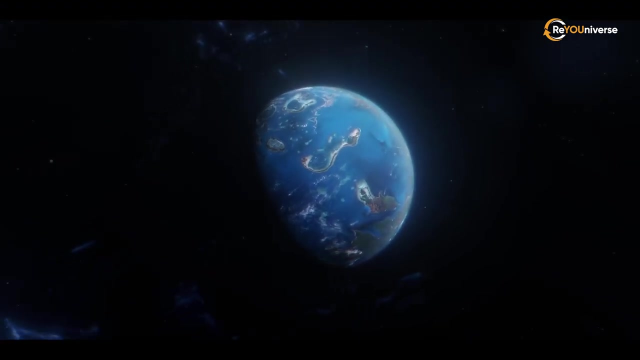 determined to be caused by a passing plane. Anyway, OSMA was the first real project that was searching for extraterrestrial radio signals. 11 Years Later, In 1971, NASA for the first time funded a SETI project. In the final report, the team 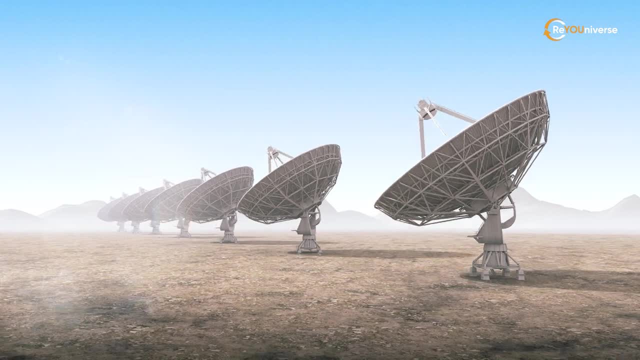 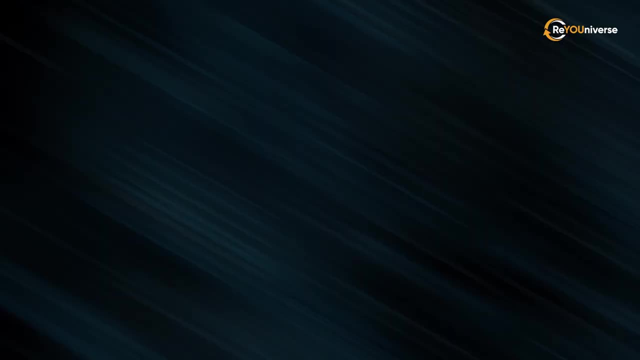 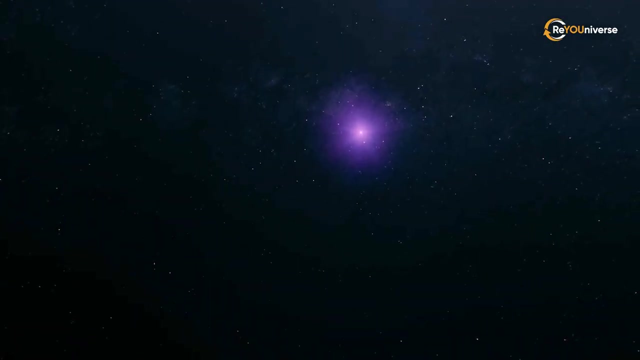 of the study suggested the construction of an Earth-based radio telescope array with 1,500 dishes. known as Project Cyclops, It was aimed to search for Earth-like radio signals at a distance of up to 1,000 light-years. Cyclops was not built due to the high-profile 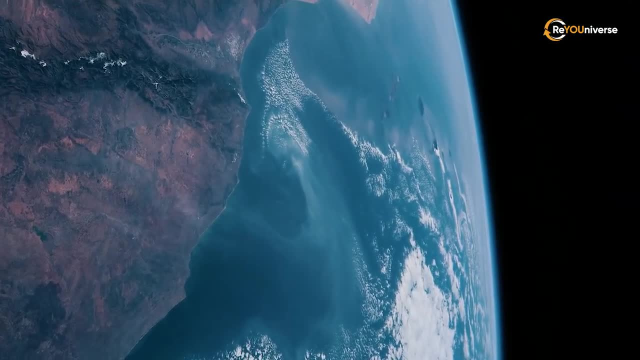 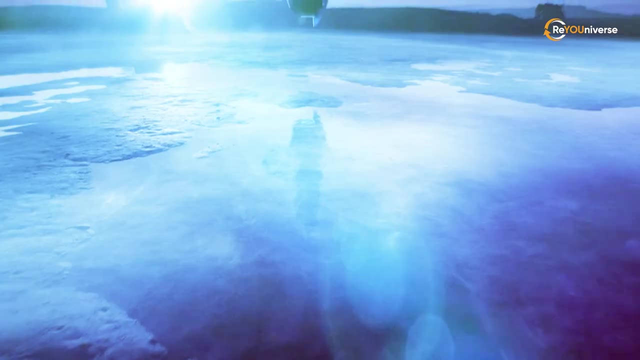 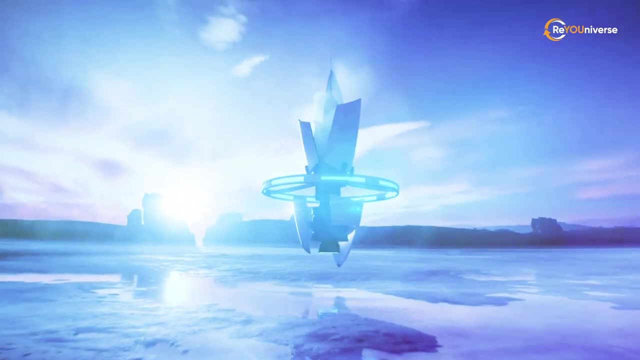 price of the project. At that time its creation would have cost around 10 billion dollars. Anyway, the report had a very important role in the history of the search for other civilizations. It created the basis for future SETI projects. We can't say that we don't receive anything. 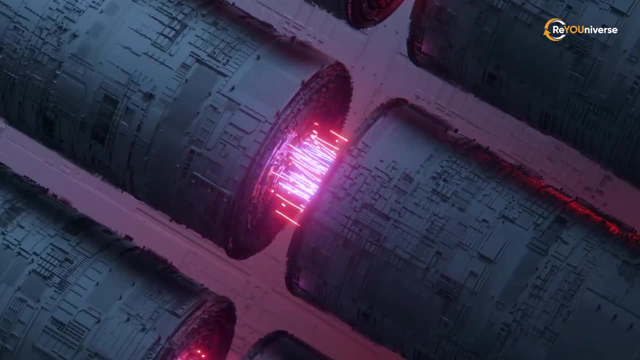 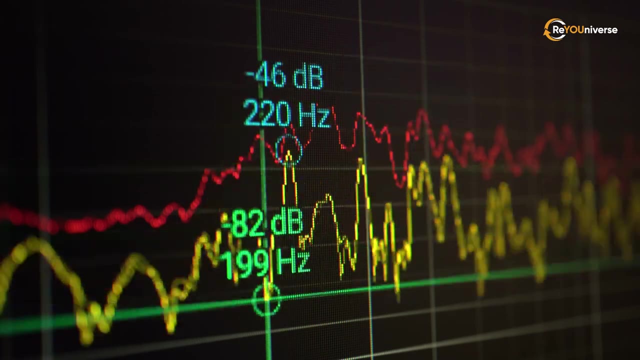 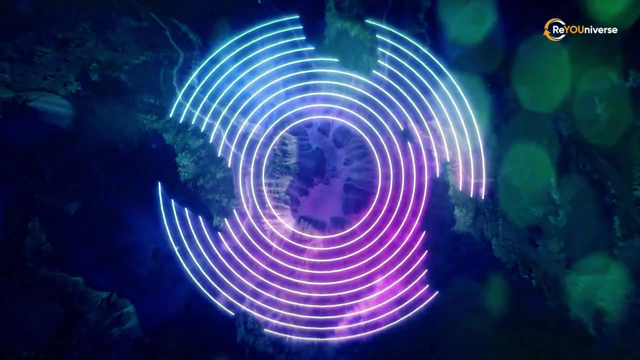 interesting from space. Sometimes we do get some strange signals, but we still cannot understand their structure. Most of them resemble the signals with which the military listens to near-Earth space. All countries have a missile defense system and it constantly monitors the passage of satellites. 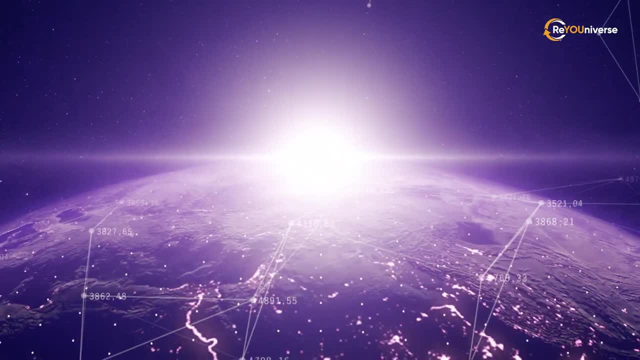 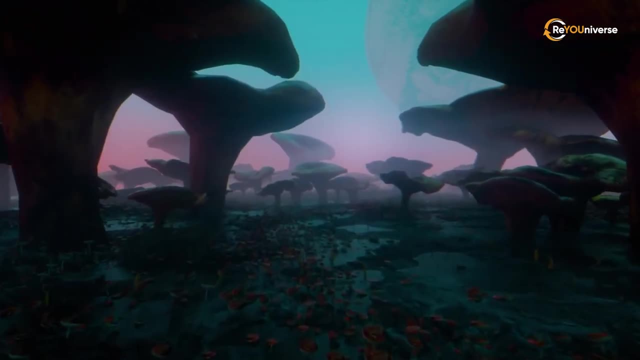 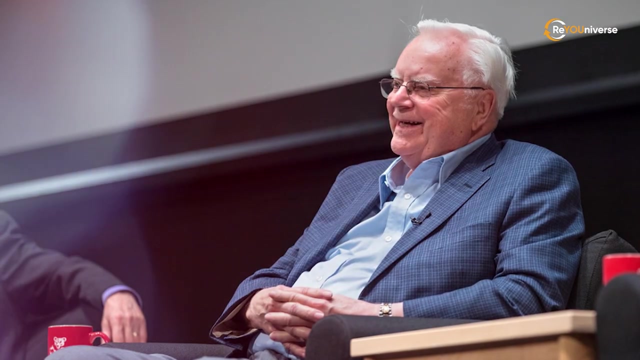 And these radio pulses are most similar to the signals that we receive. Maybe they also have anti-satellite systems. Well, we can't be really sure about anything in this case. But let's go back for a moment to Frank Drake. In the early 60s he came up with the famous Drake's equation. 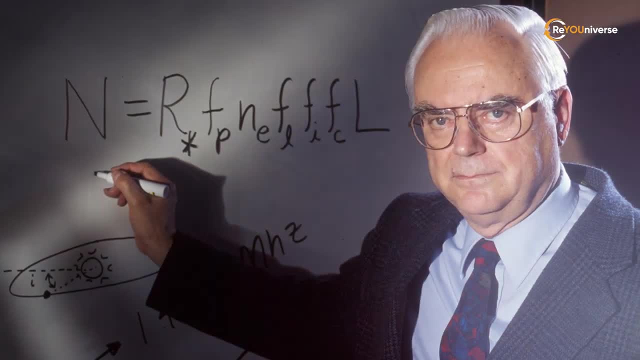 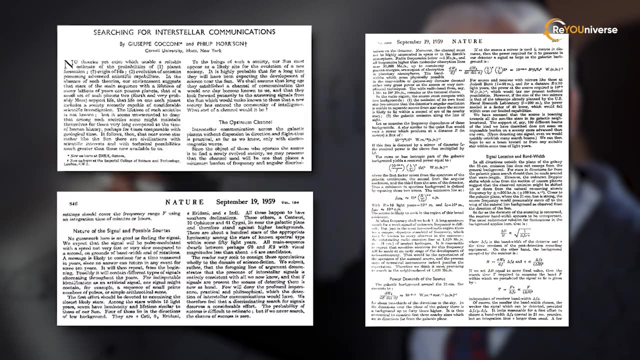 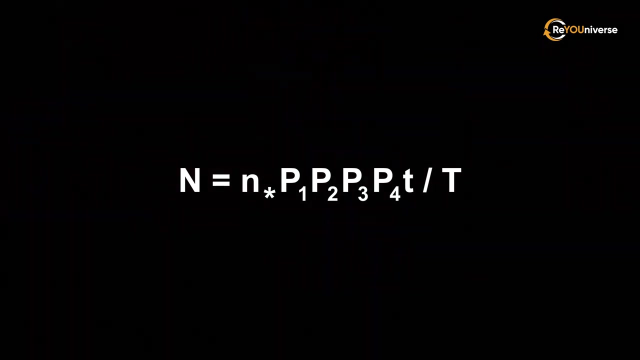 Although it's worth noting that the idea of it was formulated in Caccione's and Philip Morrison's article published by The Nature magazine back in 1959.. Anyway, what is this equation about? Well, scientists realized that the search for extraterrestrials in the universe 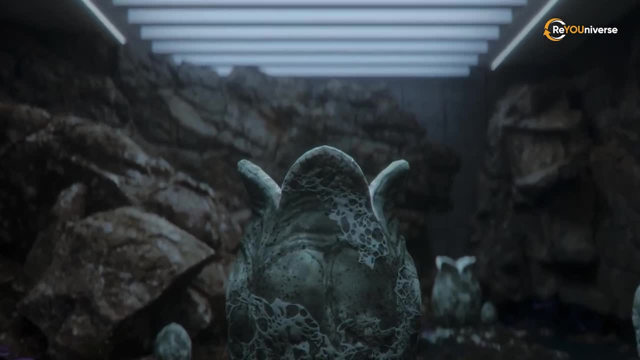 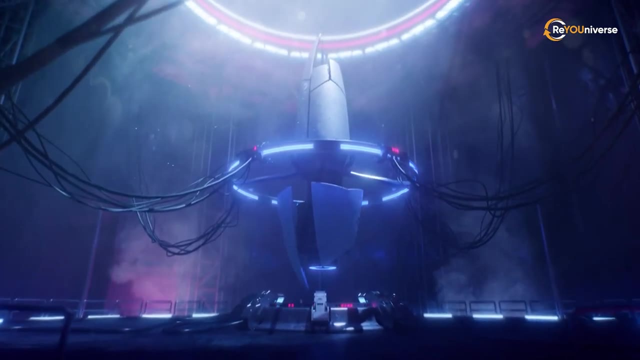 was a very complex one, And the idea of extraterrestrial civilizations is a kind of problematic matter, So it must be solved piece by piece in order to estimate the number of potential correspondents in space who are ready to keep in touch with us. 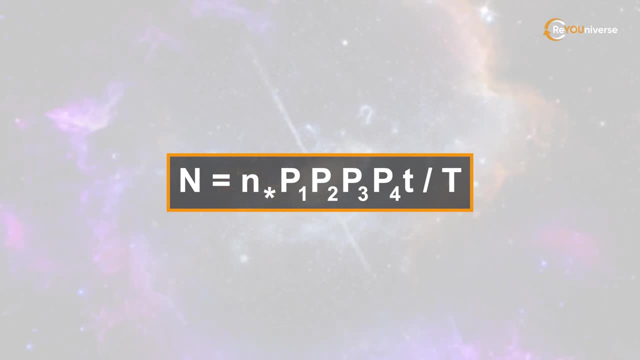 An astronomer can tell how many stars there are approximately in the galaxy. Also, he can tell how many of them have planets. Of course, somewhere there may be a civilization, But this is still not enough. It is necessary to single out the planets. 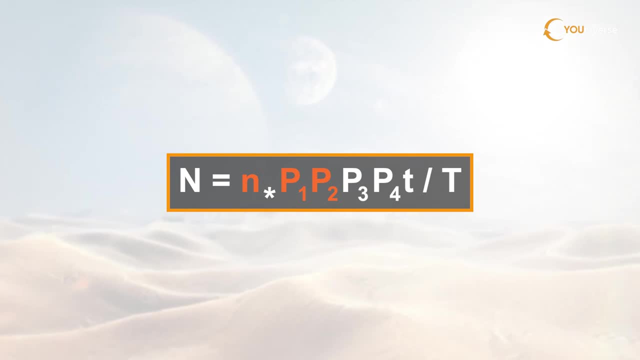 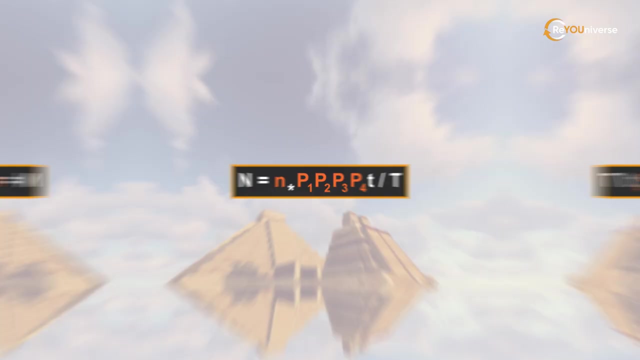 where the conditions for life are similar to those on Earth, Then we need to decide what is the likelihood that life there will reach an intellectual level and whether the intelligent civilization will get to the technical state with the possibility of contact. For example, the Aztecs were quite civilized. 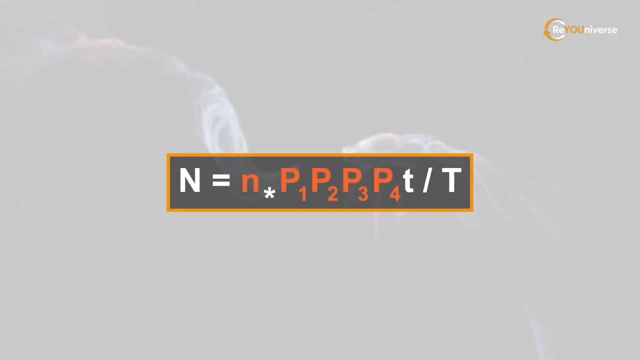 but they did not have radio equipment. And well, the most important thing is whether something in our civilization wants to make contact. And finally, we should consider the ratio of the two-existence duration of a technically advanced civilization to the age of the galaxy. 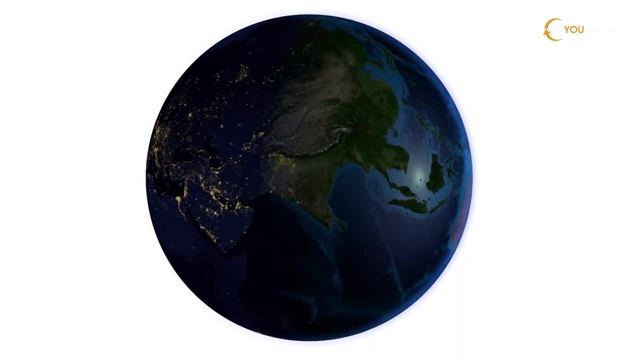 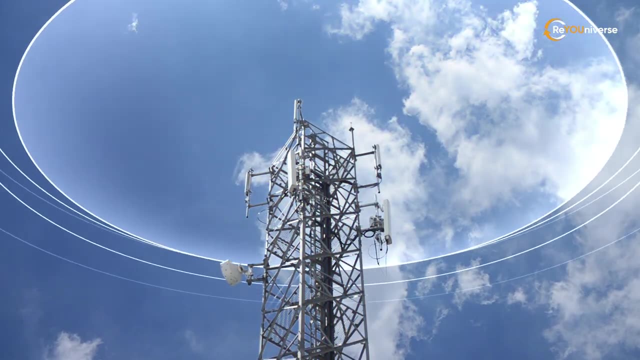 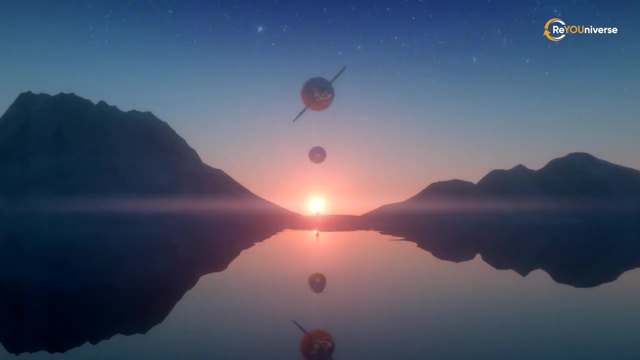 Wait what Well. take our civilization as an example. At the beginning of the 20th century we invented the radio. By the middle of the 20th century, radio technology had become sufficiently developed to support interstellar communication, But in the same years. 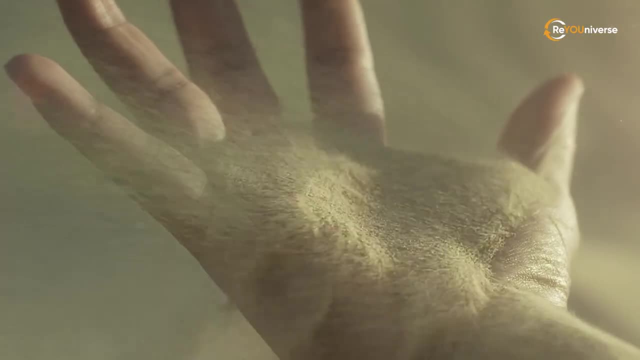 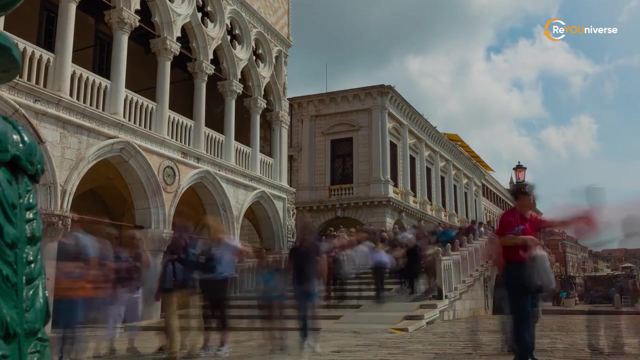 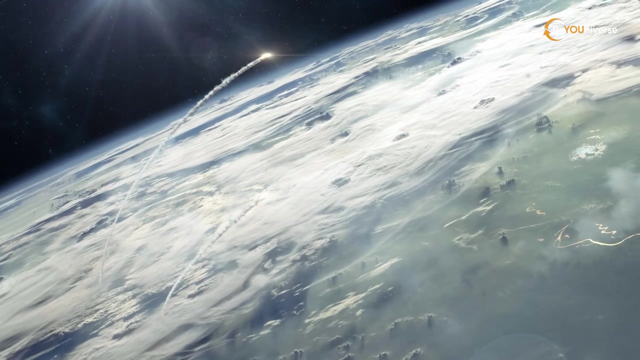 atomic and thermonuclear weapons appeared which could actually destroy our civilization. And the question is: how long does the period last when civilization has already reached the level of interstellar communication but has not yet destroyed itself? It can be a very small ratio. 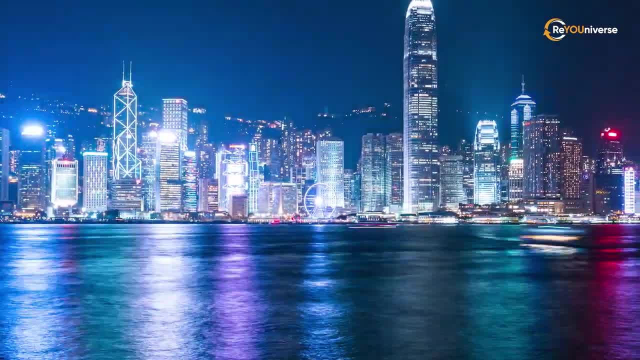 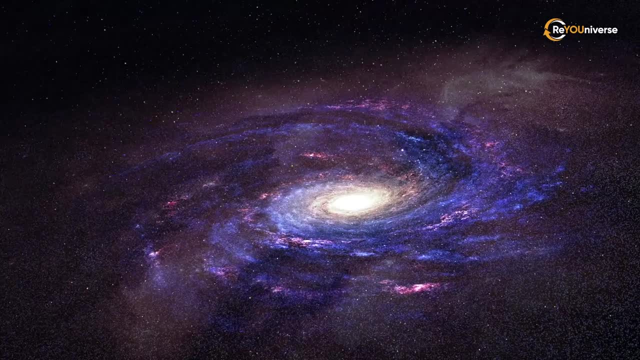 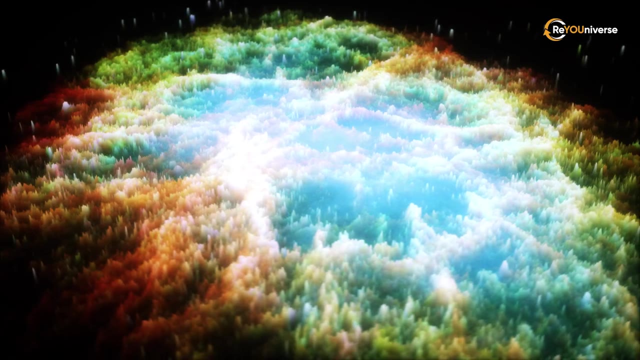 For example, in our case, we have not lived even 100 years in this period and our galaxy has existed for more than 13 billion years. The Drake equation can give a very wide range of values depending on the assumptions. That happens because the values used 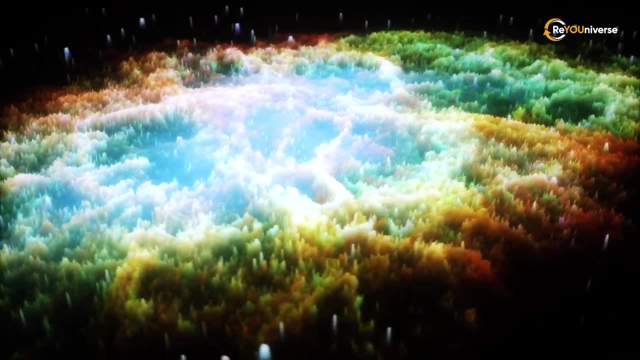 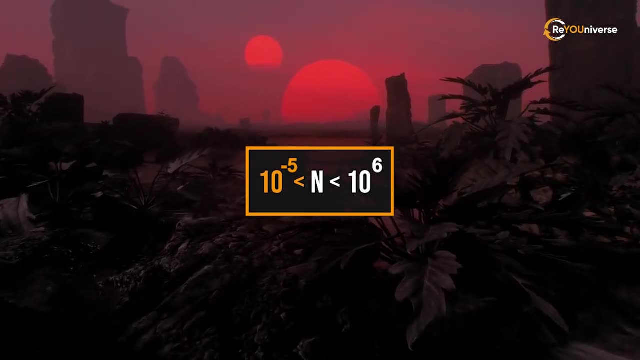 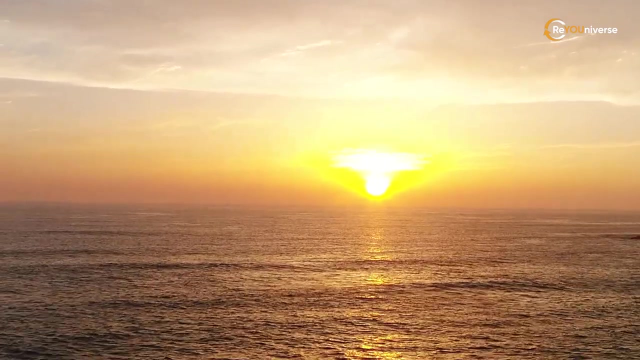 in portions of the Drake equation are not well established. Some people received final estimates of the probability near 10 to the negative fifth power. That is a value close to zero. This can only mean that there is no one in our galaxy except us. 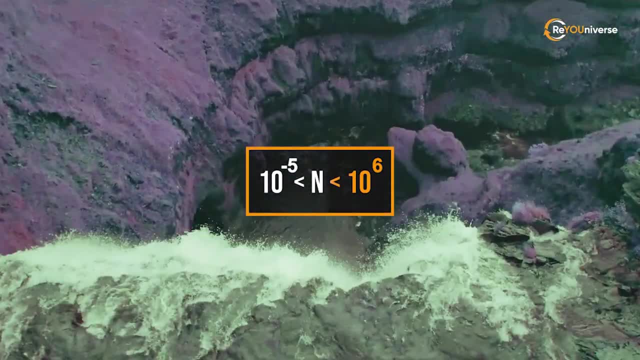 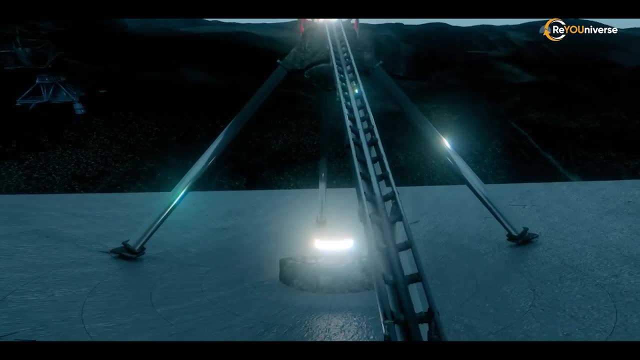 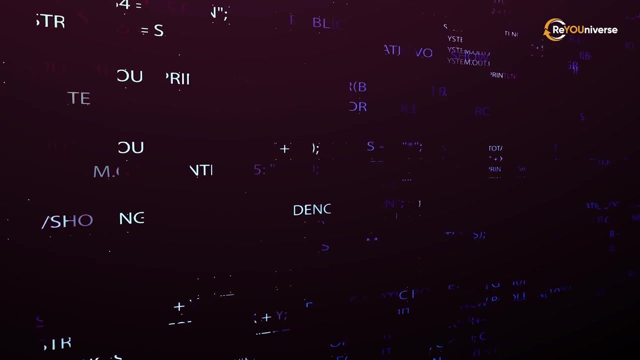 Others received large values, up to 10 to the sixth power, which gives hope that there are millions of civilizations in the galaxy who are ready for contact and are looking for it. Today, it is already possible to make this interval of estimates much more accurate. 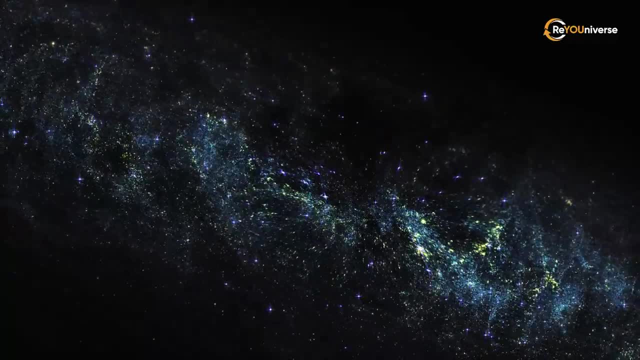 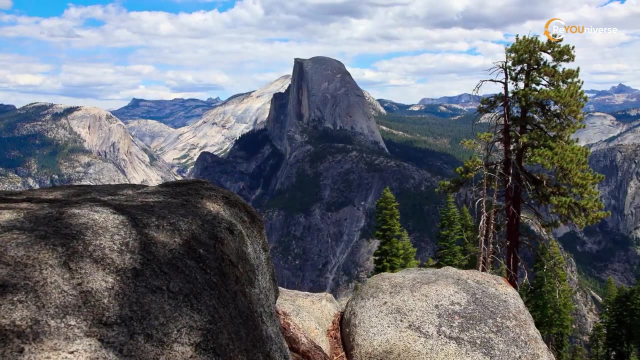 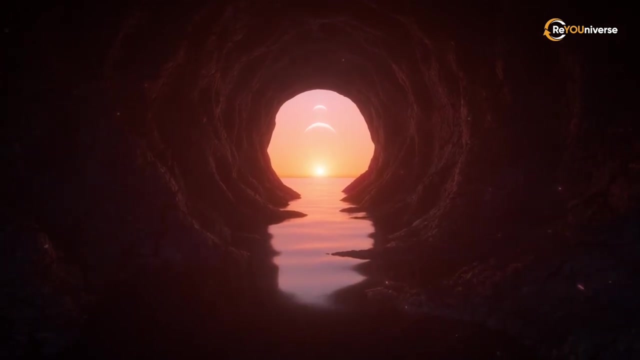 since we know how many stars are in the galaxy. Also, we learned that almost every star has a planet and most likely the next factor, which is the fraction of planetary systems with life, will be determined quite accurately in the coming decades. It is estimated that 1 in 100 planets. are similar to Earth. Anyway, the last three factors are still undefined and until we find at least one civilization, we will not know them for sure. Since 1995, scientists started to search for other civilizations and try to connect with them with even bigger enthusiasm. 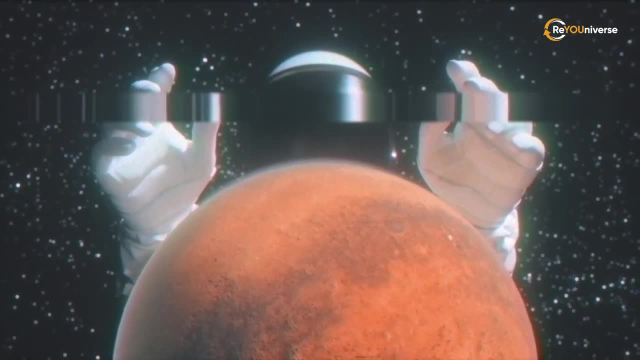 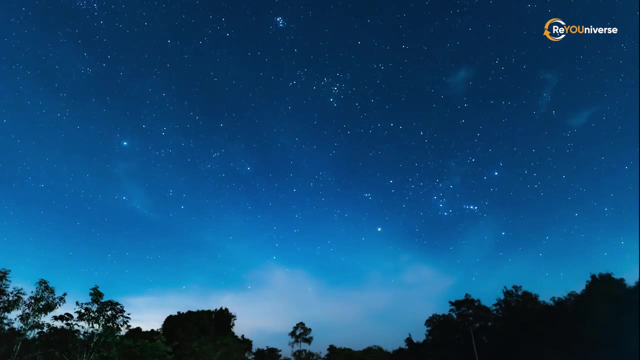 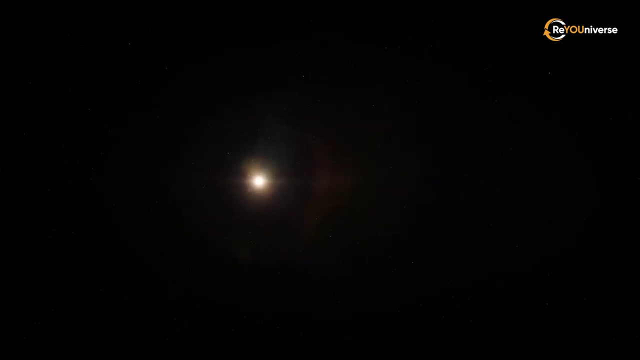 That was due to the discovery of planetary systems in other stars. At that time, no one thought that this would take place in the nearest future. There are many stars, more than 100 billion, in our galaxy alone. Astronomers never doubted that stars have planets. 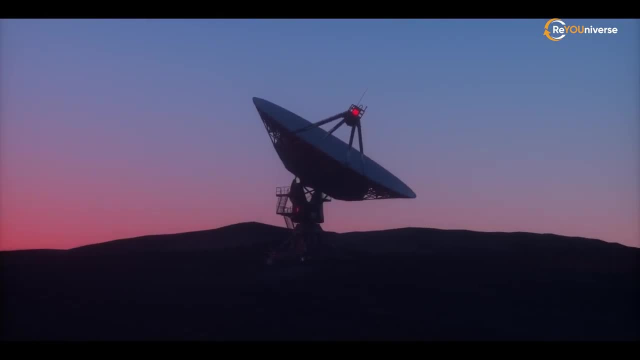 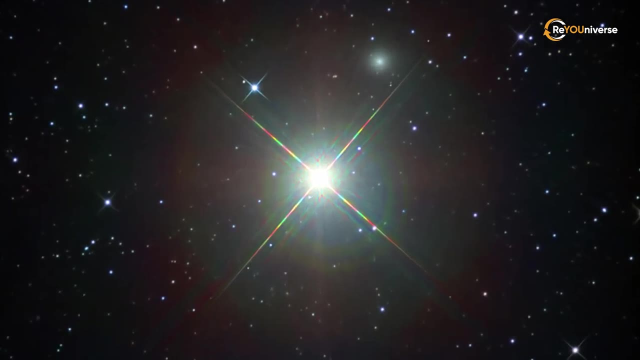 but they also did not have the technical ability to detect them. For example, this is a photo of a bright star. Its light completely blocks the area around it in a telescope and doesn't allow to distinguish anything next to it. Of course, if the brightness of the star 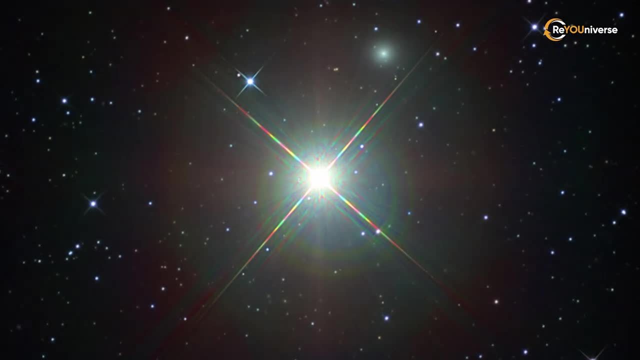 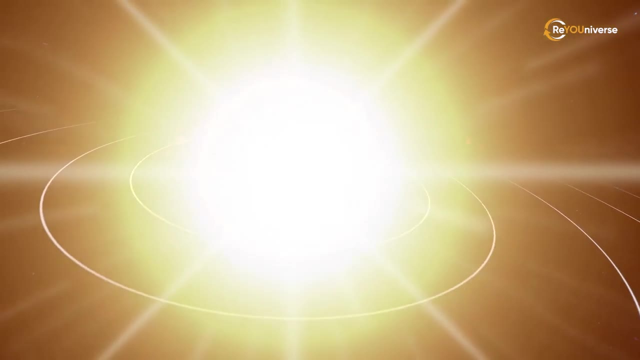 could be somehow extinguished, the planets would be visible. If you looked at our planets from the nearest stars, for example Alpha Centauri, and extinguished our Sun, then you would easily see Jupiter, Saturn, Venus and Earth. 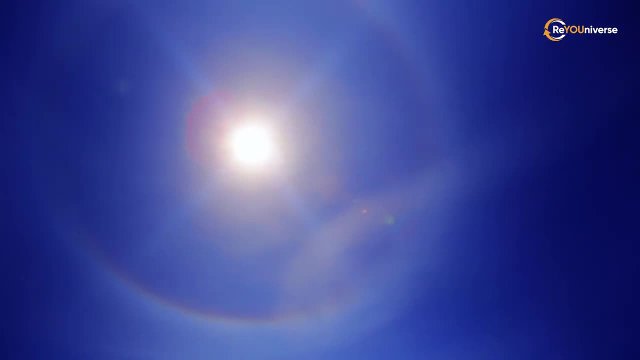 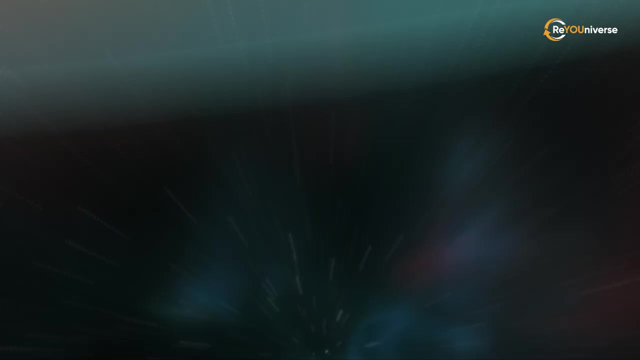 But we will never see them from afar because the star blinds us. How can we solve this? Well, there's a way, even for that. We do not see the planets, but let's take a look at the star. It cannot remain stationary. 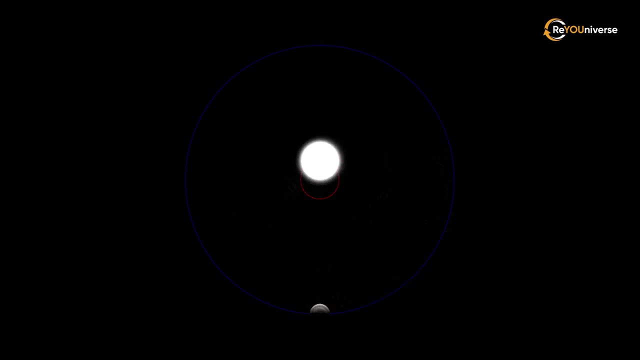 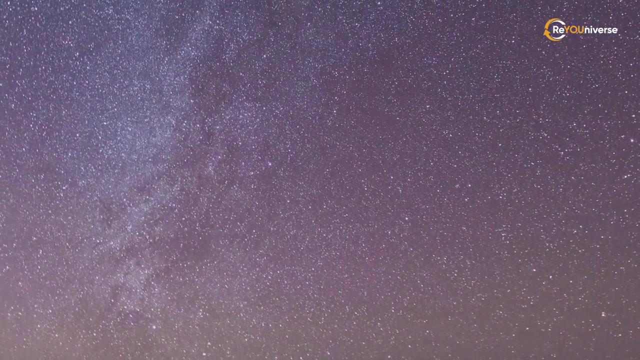 if a planet revolves around it, And this will be a sign that there is a planet there. But how can we notice the movement of a star? We see a stream of light from every star split by a prism or a diffraction grating. 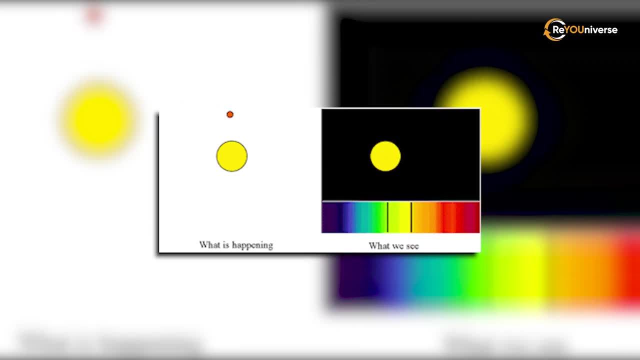 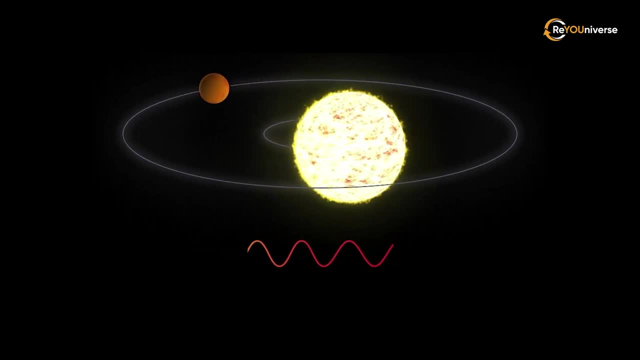 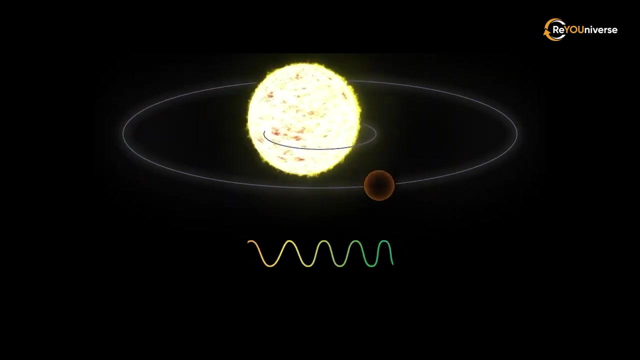 This is a spectrum. If the star is stationary, then the spectral lines stand still. If the star regularly moves, then these spectral lines will move, as due to the Doppler effect. But noticing them actually is not that easy, Why, Well? 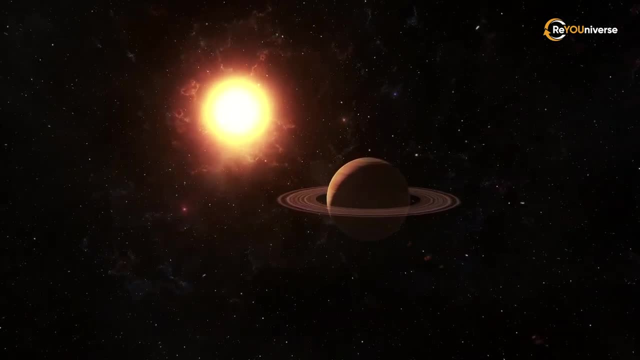 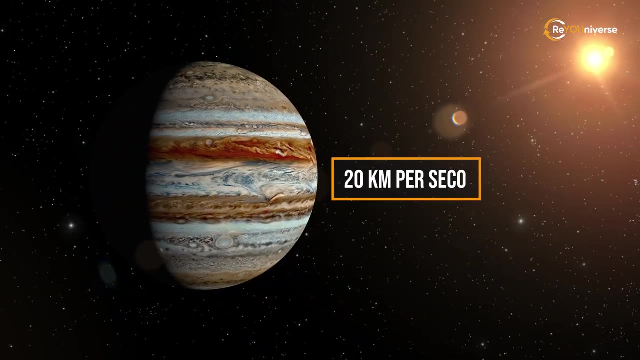 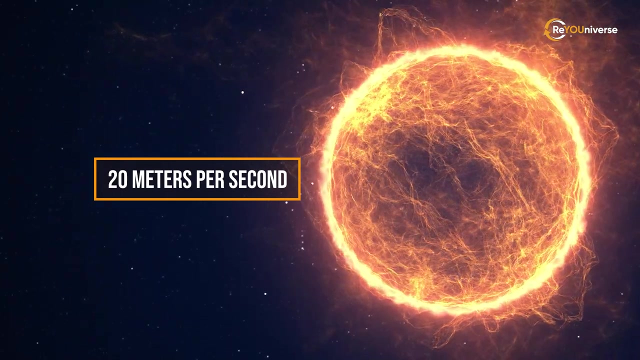 it's easy to explain on Jupiter, since it is the most massive planet in our system and therefore affects the Sun more than the other planets. Jupiter orbits at about 20 kilometers per second. The Sun is thousands of times more massive than Jupiter, which means that it has a thousand times. 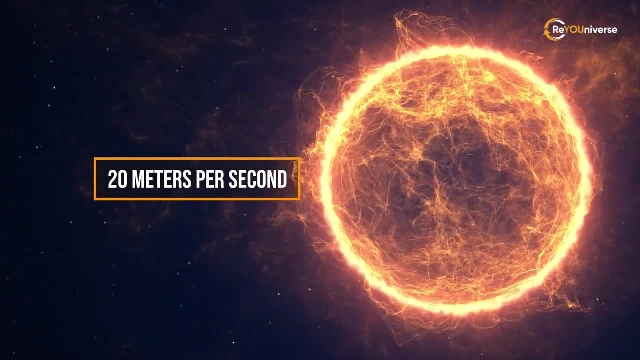 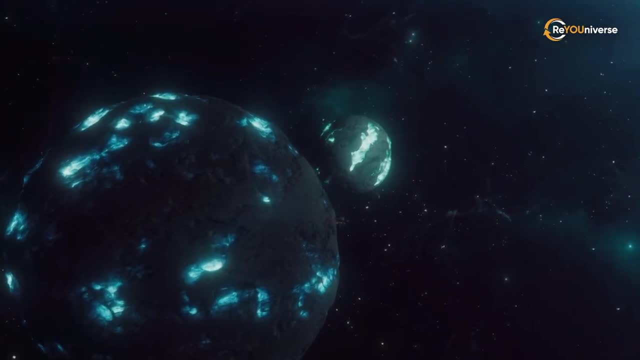 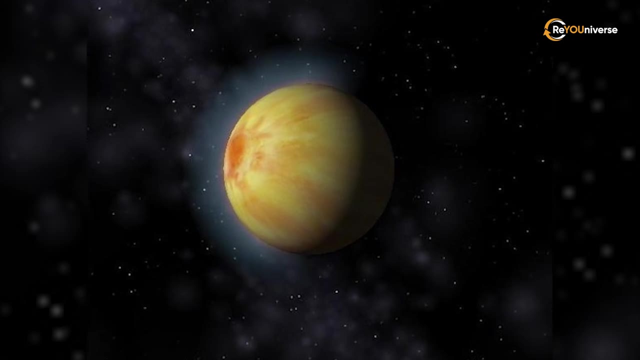 less speed. It's 20 meters per second On a cosmic scale. this is a very low speed. Anyway, scientists managed to see the movement And at the end of 1995, the long-awaited event took place For the first time. an exoplanet was discovered near star 51 in the Pegasus constellation. By the way, exoplanet is the name for the planets of the other stars. Now we find over 100 of them per year, But it turned out that it is possible. 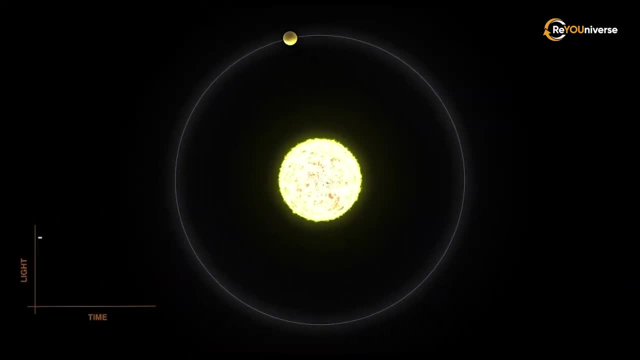 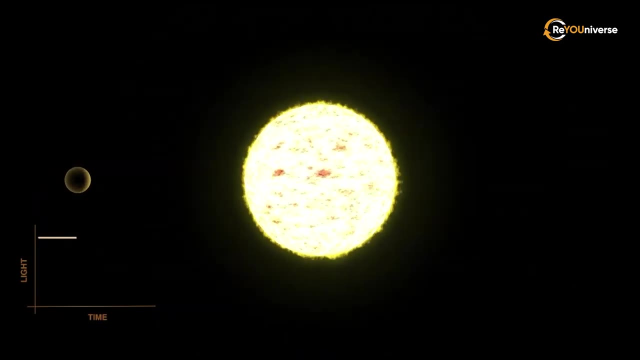 to find these planets differently. So if their orbit lies in a plane passing, from our point of view, in front of the star, then sometimes the planet will cover its star and its light will darken a little bit. for our telescopes It is especially convenient. 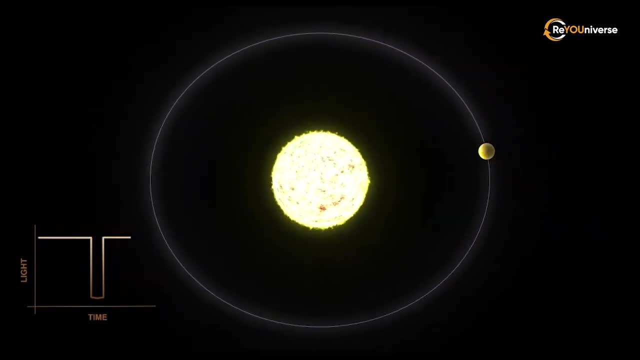 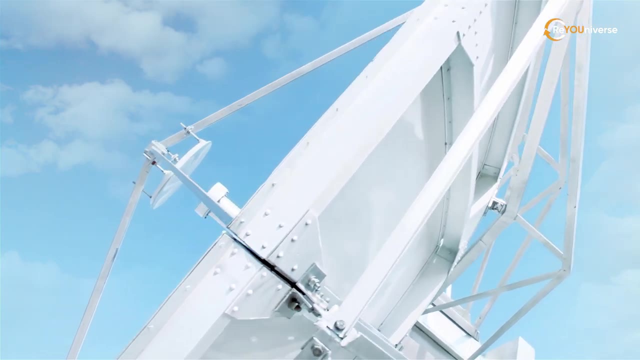 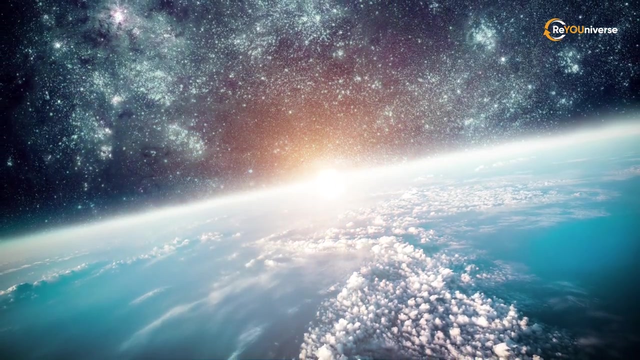 to detect such eclipses with space telescopes. This method also allows the detection of planets passing in front of the star. Moreover, it allows you to explore them. When a planet passes in front of a star, the star's light is scattered into the planet's atmosphere. 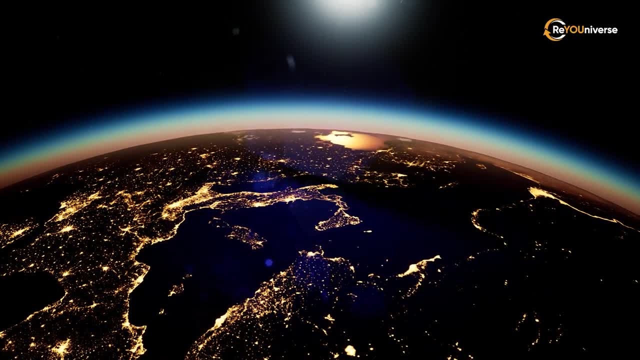 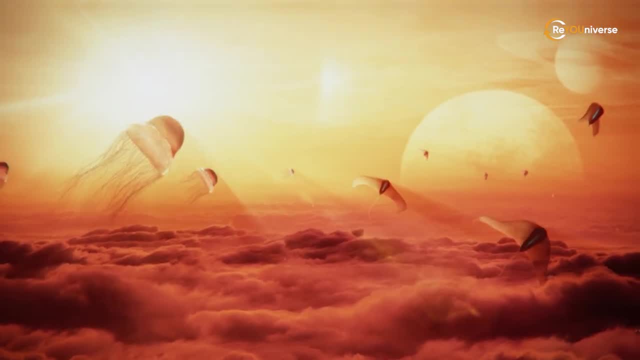 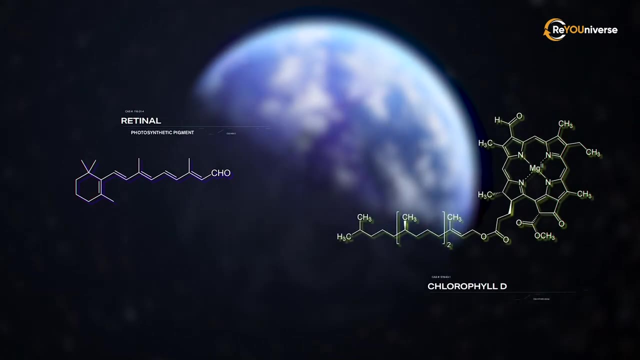 And so the light comes already with signs of the atmosphere, with some spectral lines that have arisen in the gaseous envelope of the planet. Therefore, we can study the chemical composition of the exoplanet's atmosphere. But what do we hope to find there?